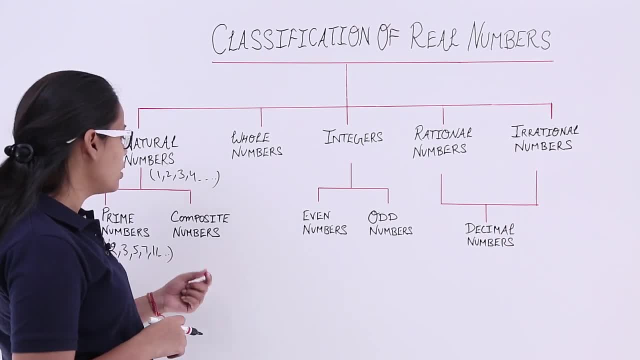 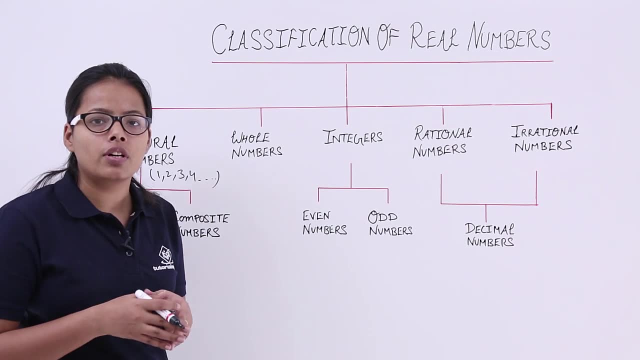 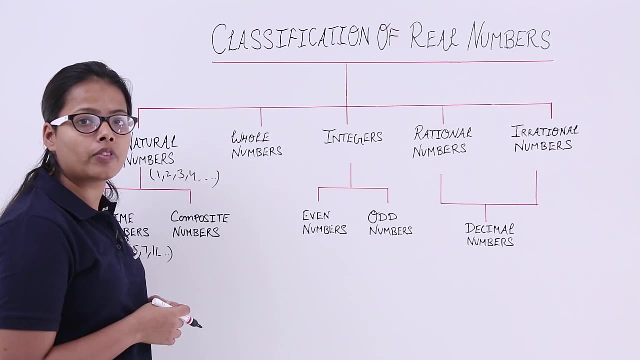 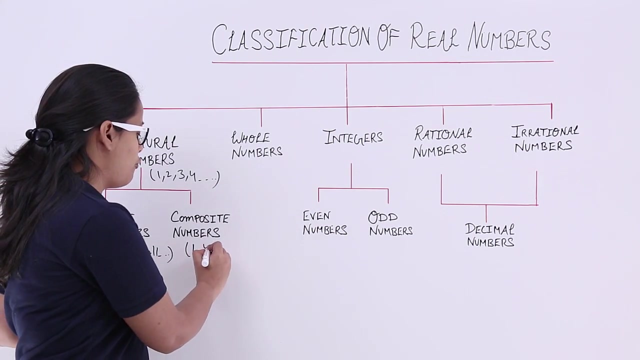 numbers comes under prime numbers. Now let's move on to composite numbers. What are composite numbers? Composite numbers are the composition of numbers and they include all the numbers excluding prime numbers, such as 1, which is not included in prime numbers, 4, which is also not included in the prime numbers, 6,. 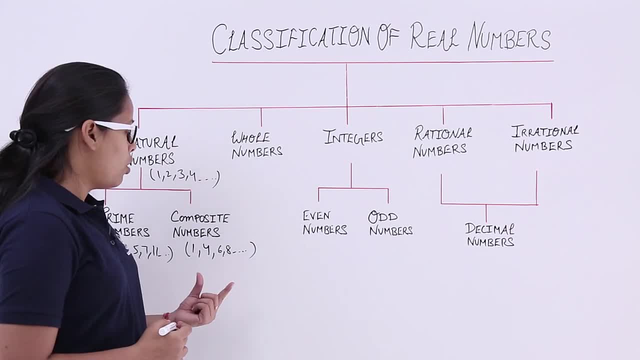 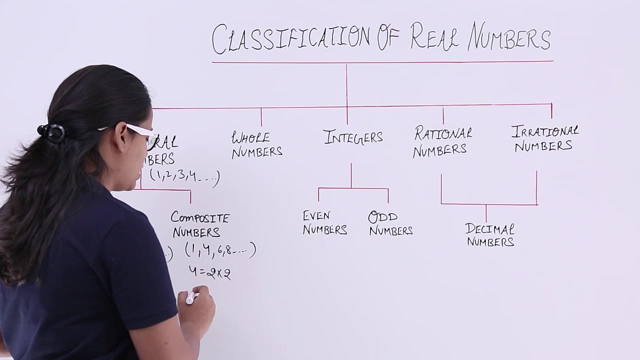 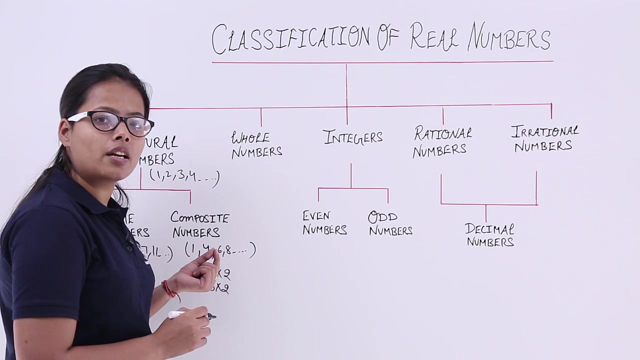 8 up to so on. All the composite numbers plus all the prime numbers give you natural numbers. So for example, 4 it is the composition of 2 into 2, 6 it is the composition of 3 into 2.. So here you can see all the numbers. under composite numbers are the composition of numbers. 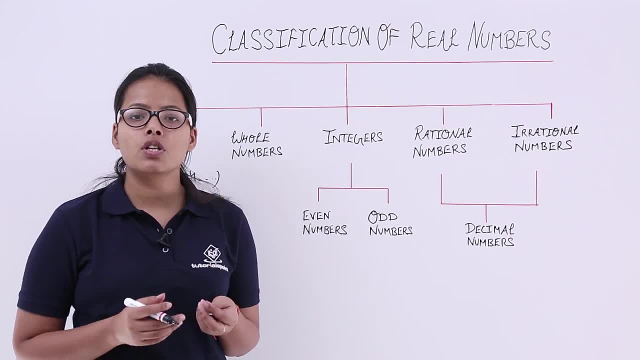 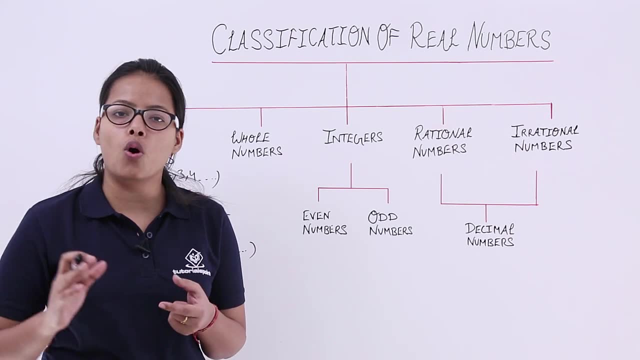 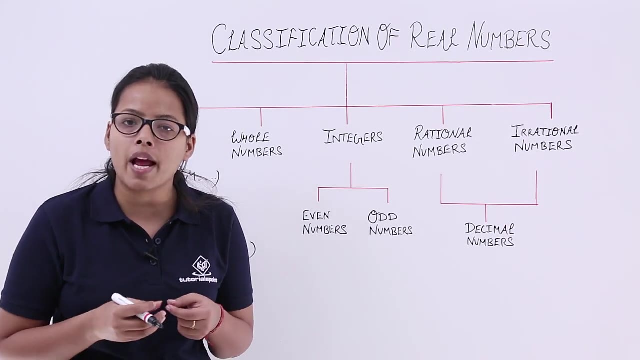 Okay, So now, what do you understand by natural numbers? All the counting numbers which you have learnt in earlier classes: 1, 2,, 3, 4 up to so on. These are the natural numbers, which are further divided into prime numbers and composite numbers. What are prime numbers? 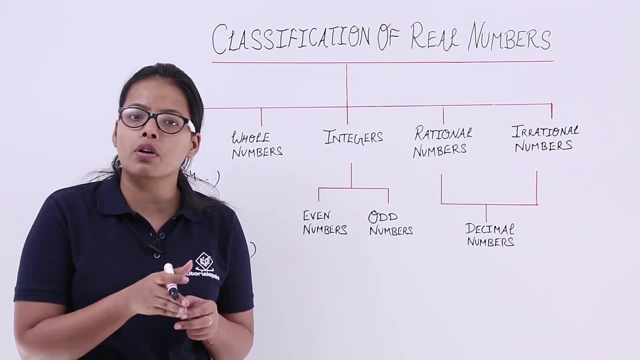 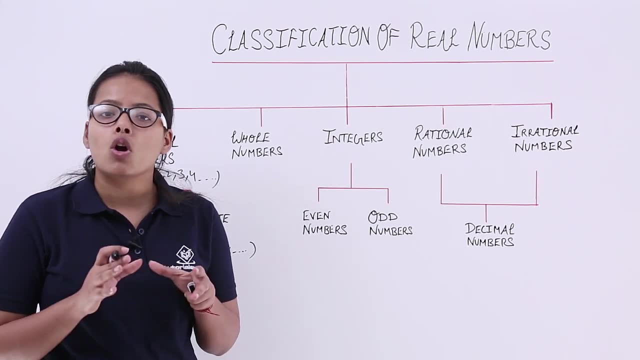 Prime numbers are those numbers which are divisible by its own numbers. So these are its own number and 1. But it is not divisible by any other number. And what do you understand by composite numbers? Composite numbers are the composition of numbers. Okay, For example, 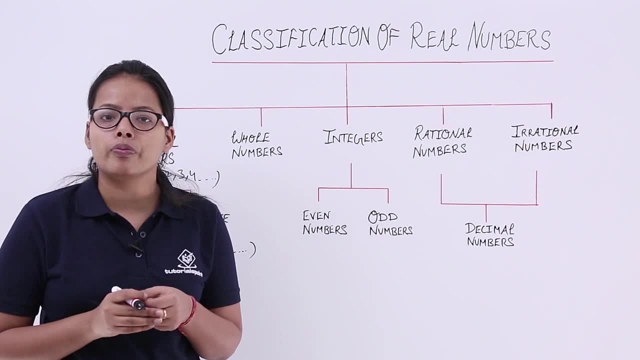 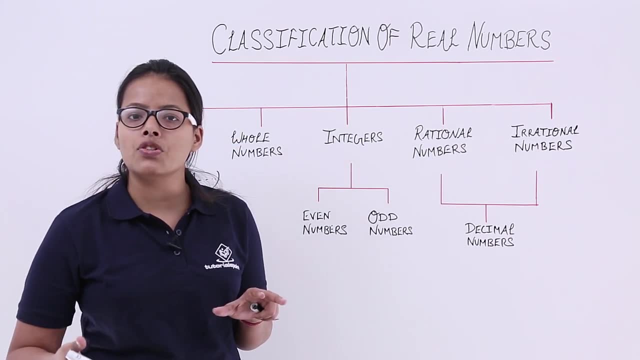 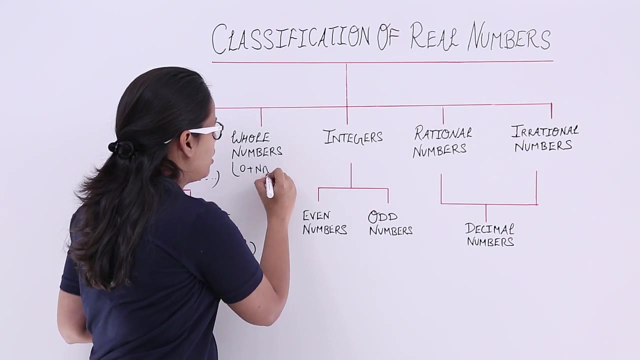 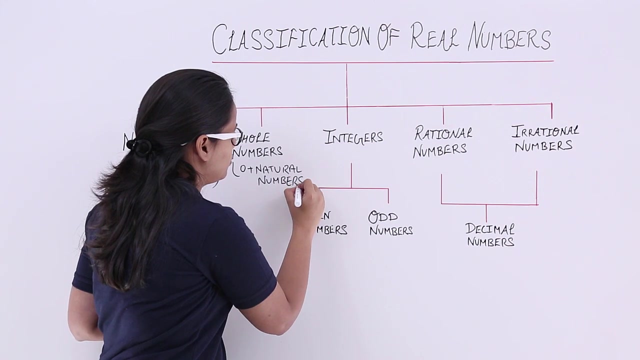 4. it is the composition of 2 and 2.. Okay, Now let's move on to whole numbers. Whole numbers are all the natural numbers, including 0. How 0 plus all the prime numbers. So this is 0 plus all the natural numbers. And how can you remember whole numbers? By keeping. 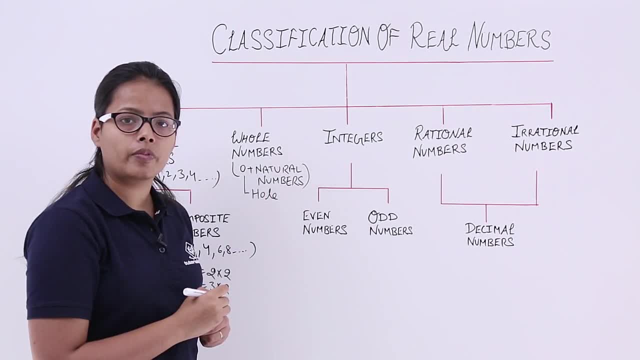 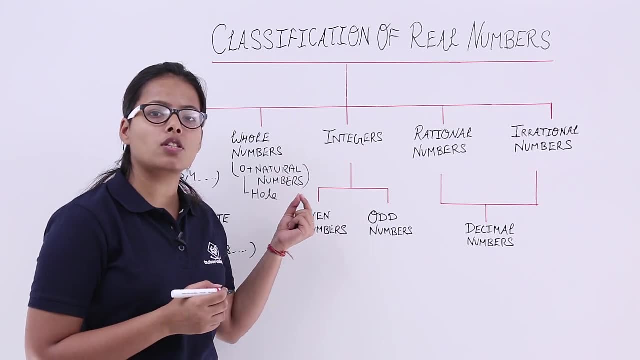 in mind 0 as whole, As the title is whole. Okay, So what numbers are included in a whole? numbers 0 plus all the natural numbers, 0,, 1,, 2,, 3,, 4, up to so on. Okay, So what numbers? 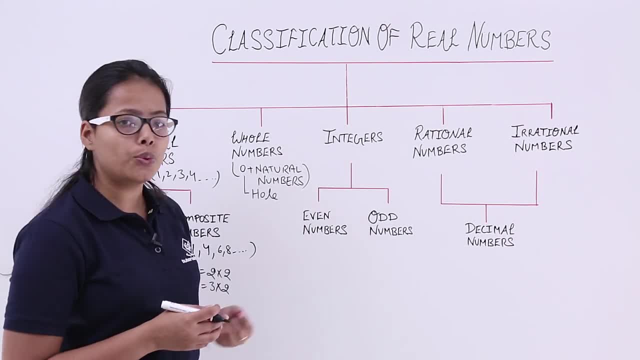 are included in a whole numbers 0, plus all the natural numbers 0,, 1,, 2,, 3,, 4, up to so on. Okay, So now let's move on to integers. What are integers? All the positive whole. 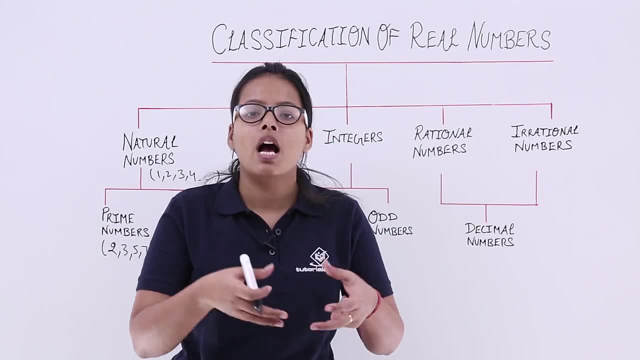 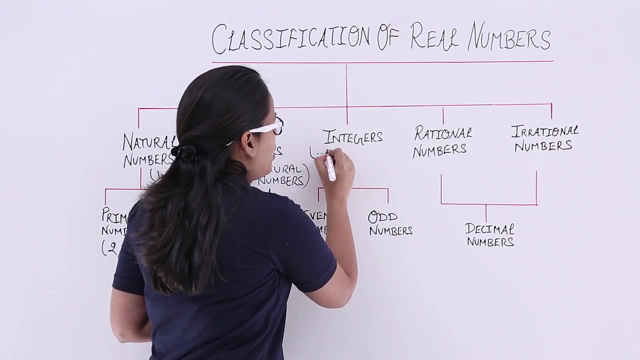 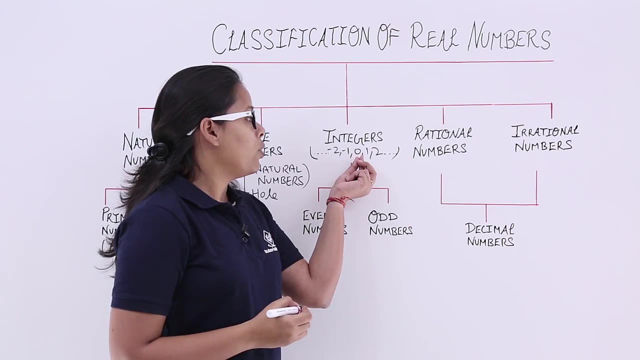 numbers, as well as all the negative of the whole numbers are the integers Okay, Such as minus 2, minus 1, 0, 1, 2 up to so on 1 plus its brother, minus 1.. 2 plus its brother. 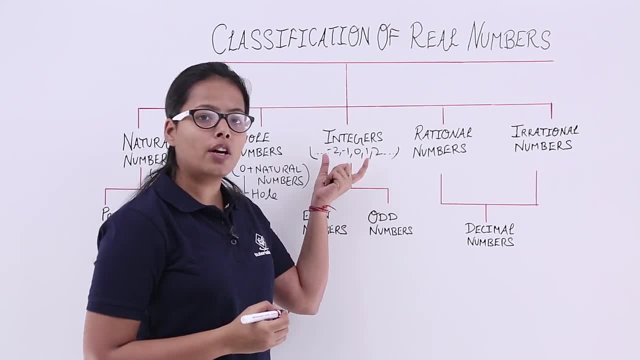 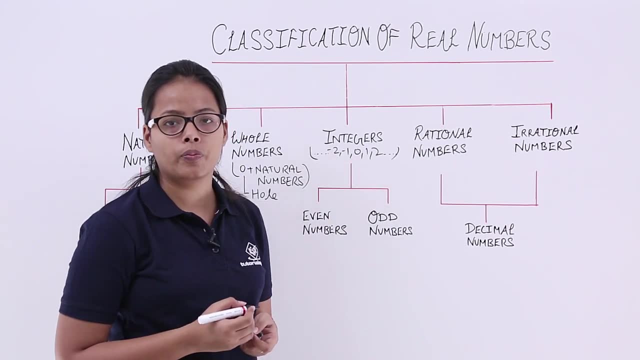 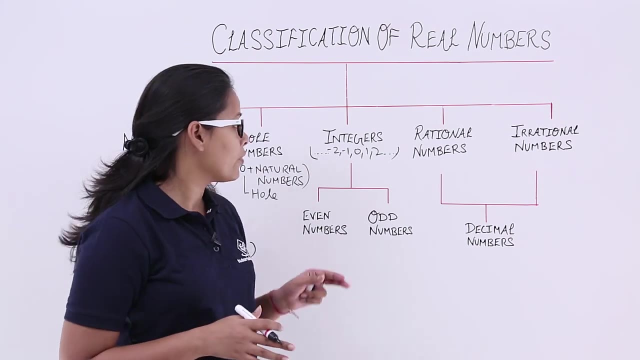 minus 2.. That's how you'll remember. So there are 2 brother 1 minus 1, 2 minus 2, 3 minus 3, including 0.. Okay, So these numbers are integers. That's how you'll remember. Okay, So integers are. 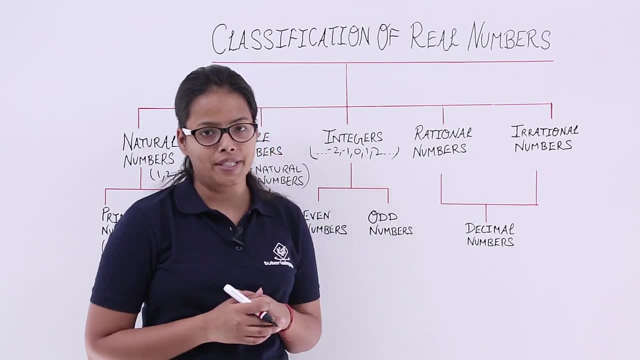 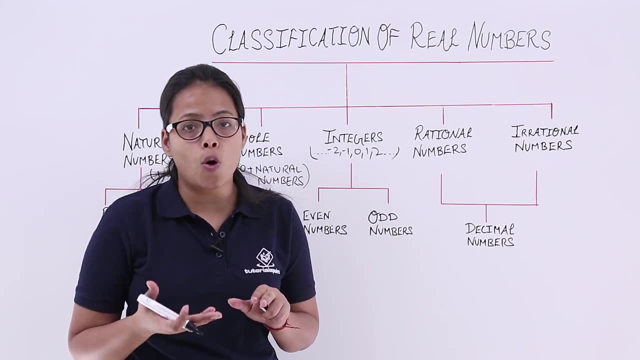 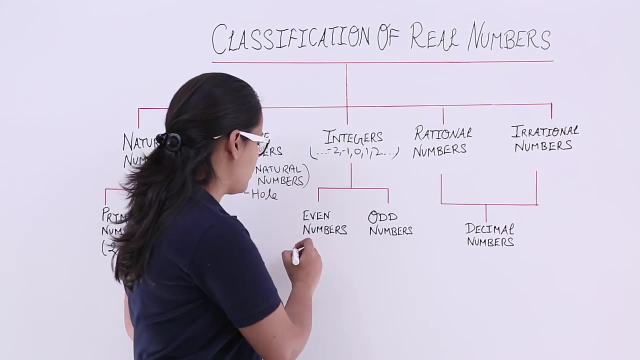 further classified into even numbers and odd numbers. Even numbers are all those numbers which are divisible by 2.. And those numbers which are not divisible by 2 will come under odd numbers. So let's see what are the even numbers Minus 2, 0, 2, 4, up to so on 2 minus. 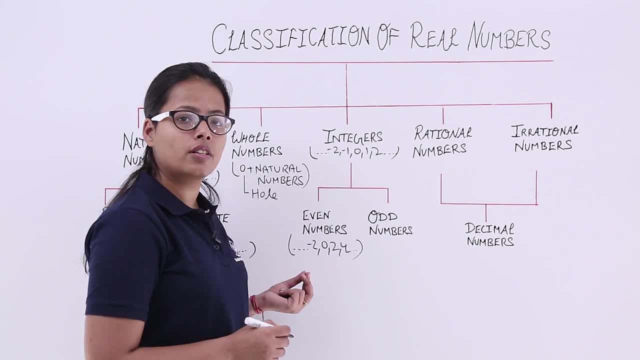 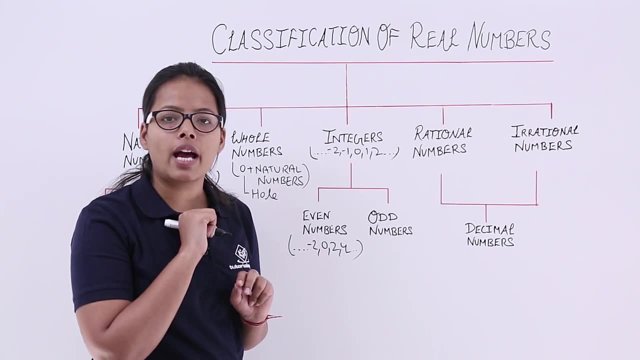 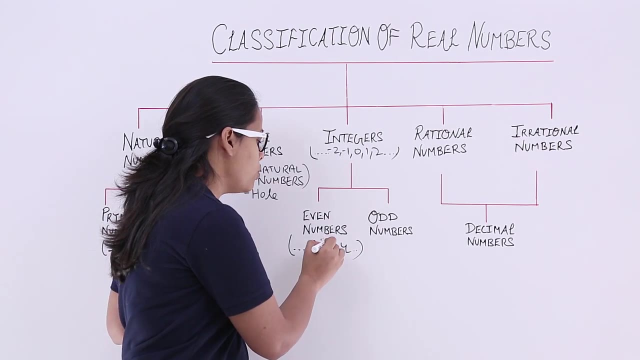 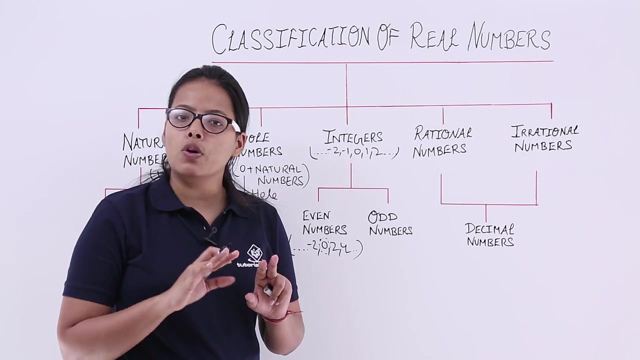 2, 4 minus 4, 6 minus 6.. All these numbers are completely divisible by 2.. There will be remainder. You'll be getting the remainder as 0, because these numbers are completely divisible by 2.. Now you must be wondering why 0 is an even number, because 0 is divisible by 2.. 0 is divisible. 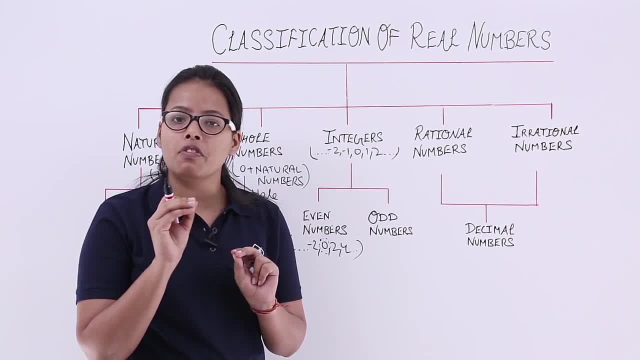 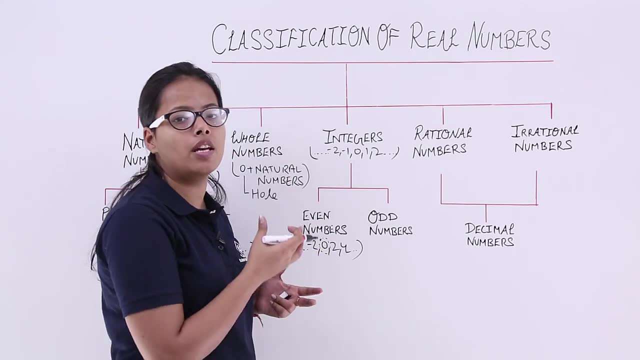 by all numbers, but you need to see if it is divisible by 2, then it will come under even category, Because 0 is divisible by 2, that's why 0 is an even number. Okay, So now let's move on to odd numbers. 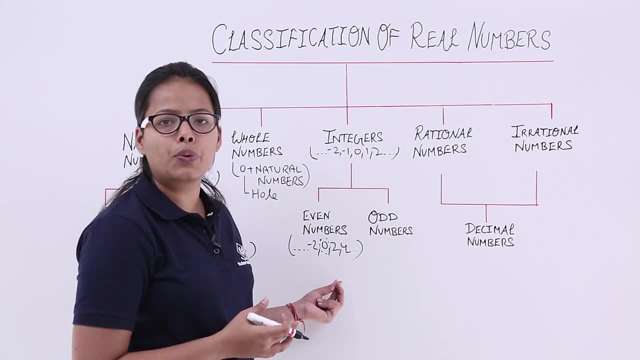 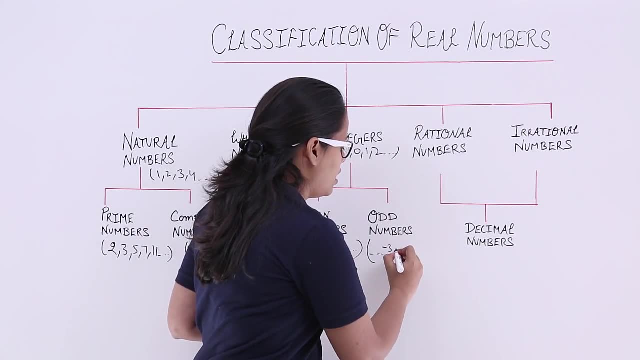 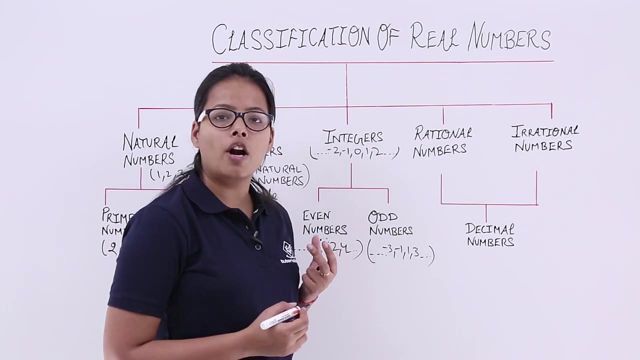 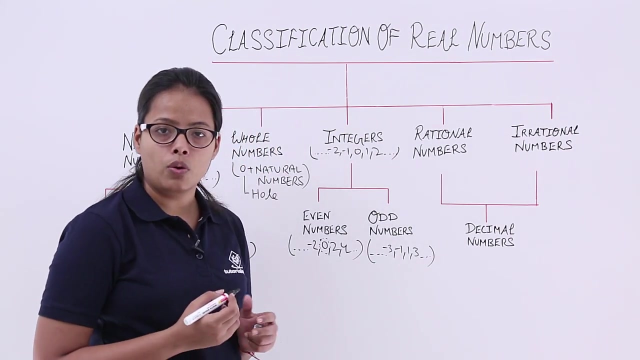 All those numbers which are not included in the range of even numbers will come under odd numbers, such as minus 3, minus 1, 1, 3.. So, brothers, of all the odd numbers, 1, minus 1,, 3, minus 3,, 4,- sorry- minus 5, 5.. Okay, So all these are odd numbers. So now what? 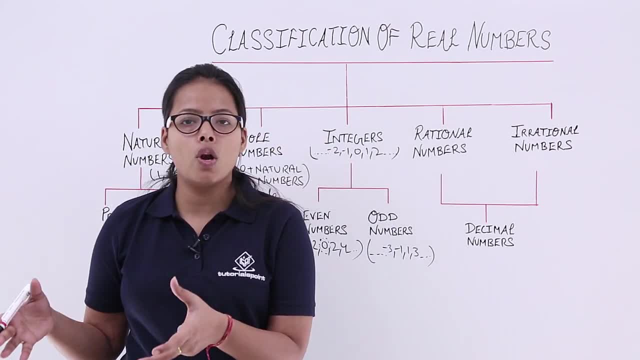 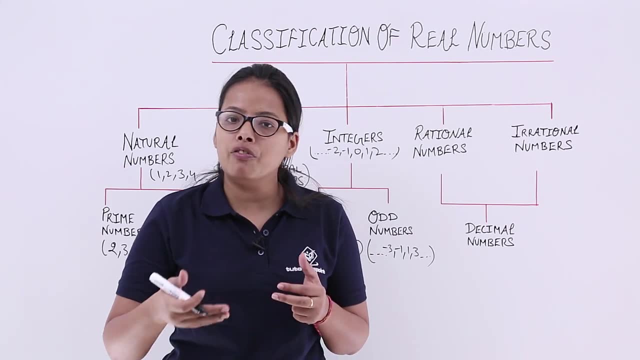 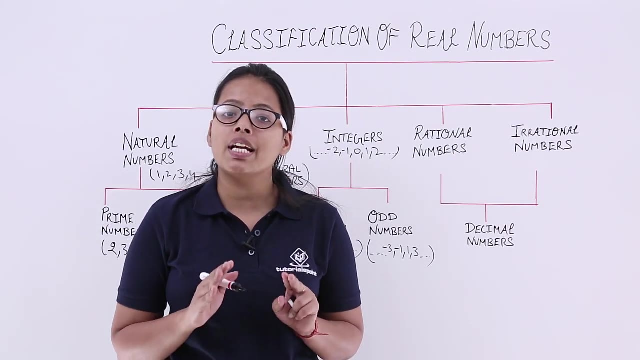 do you understand by integers all the positive whole numbers as well as all the negative. of these whole numbers are the integers, which has been further subdivided into even numbers and odd numbers. Even numbers are all those numbers which are completely divisible by 2. Odd numbers are those numbers which are not 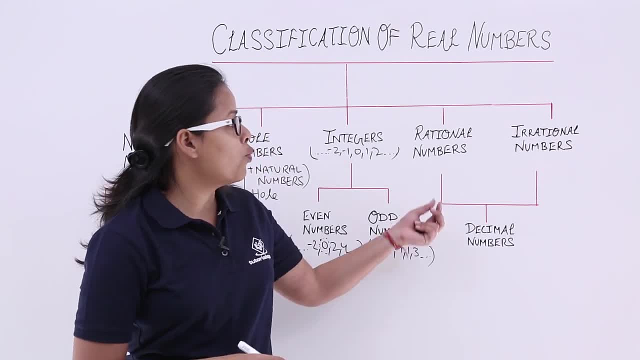 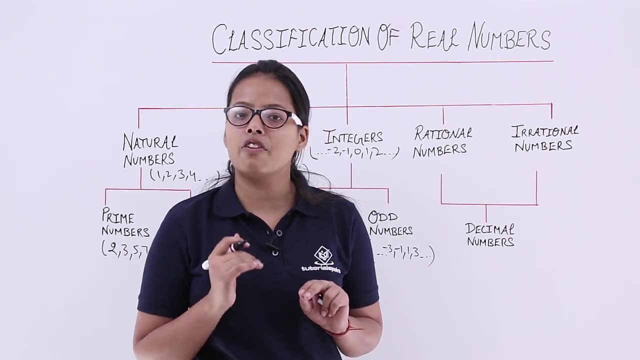 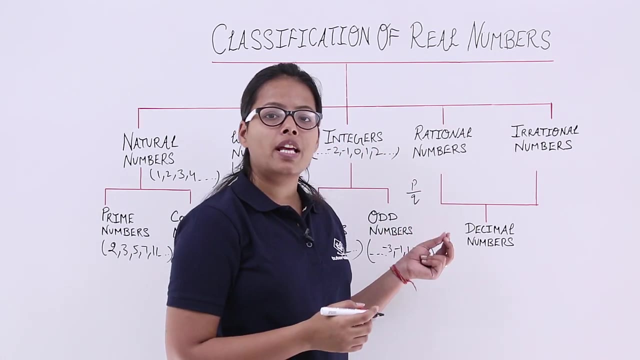 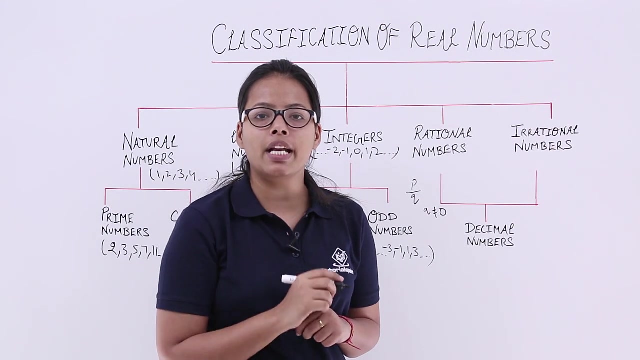 divisible by 2.. Okay, so now let's move on to rational numbers. Rational numbers are always represented in the form of integer by integer, fraction, How P by Q, where P as well as Q, both are integers, but the value for Q should not be equal to 0.. Keep in mind: value for Q should not. 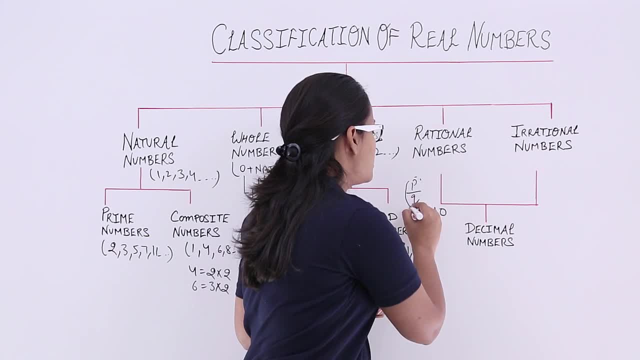 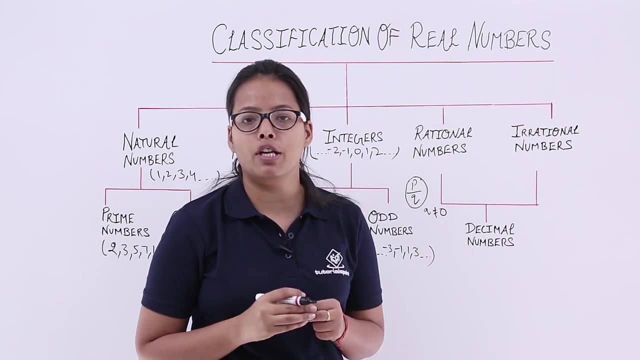 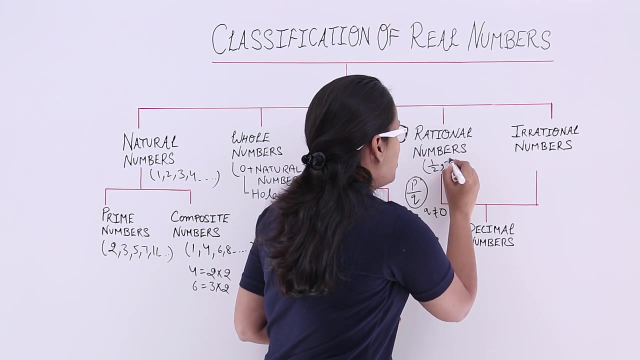 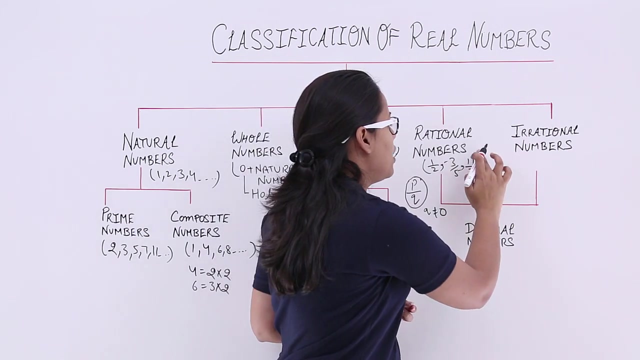 be equal to 0. If value for Q is 0, then the value for P by Q will become undefined. There won't be any definite value for this. Okay, so now let's see, For example, 1 by 2 minus 3 by 5, 11 by 7.. So all these numbers are rational numbers. 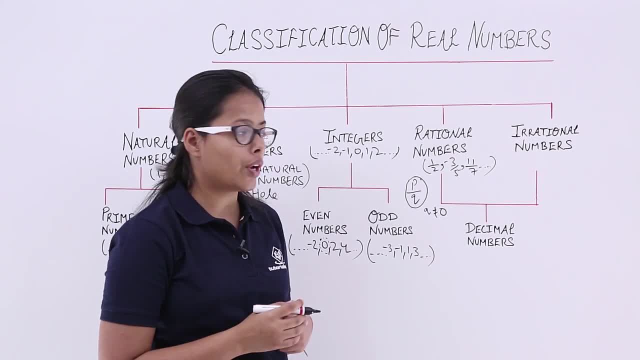 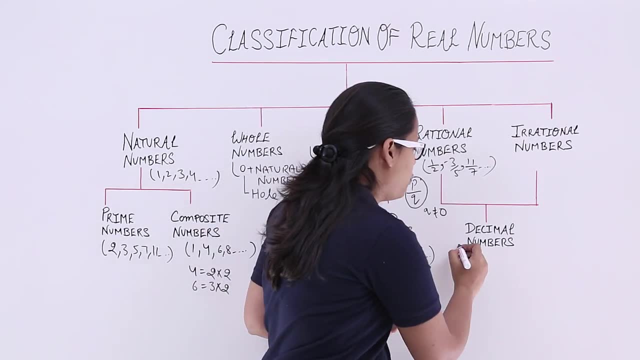 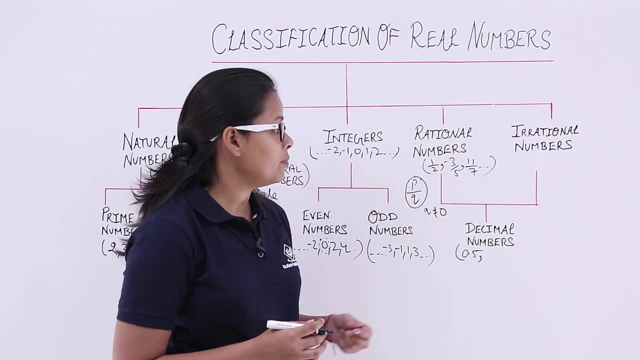 There are infinitely many rational numbers. Okay, when you expand these numbers, you will get decimal numbers. When you divide 1 by 2, the value for 1 by 2 will be 0.5, which is a decimal number. When you divide minus 3 by 5, what you'll get, You'll get. 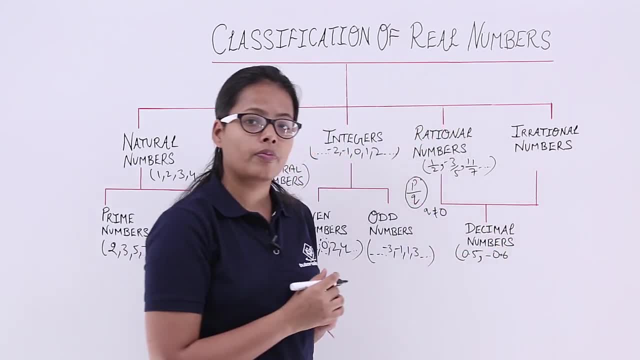 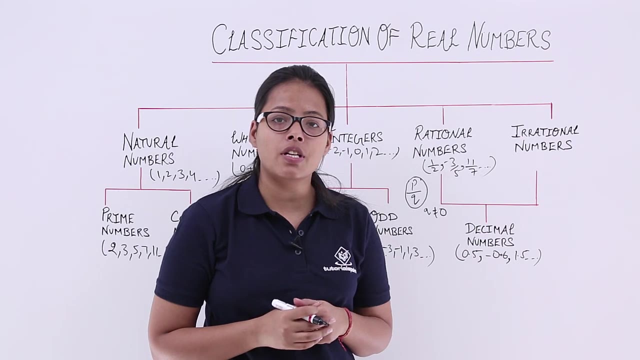 minus 0.6.. If you divide 11 by 7,, what you'll get? You'll get 1,, 5, up to so on. Okay, So these all are the decimal number. What do you understand by rational numbers? Rational- 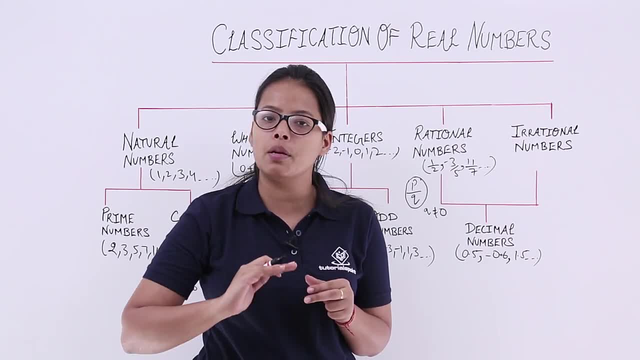 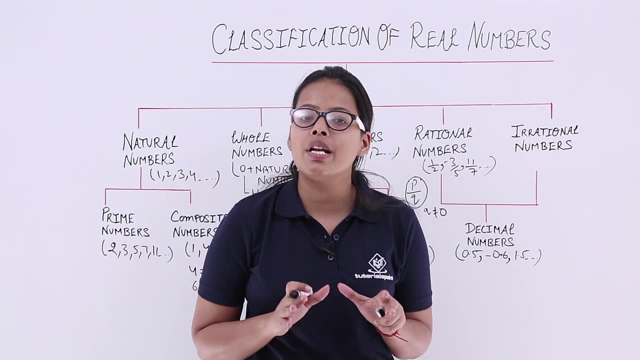 numbers are all those numbers which can be represented in integer by integer fractional form. Okay, So now let's move on to irrational numbers. What do you understand by irrational numbers? Irrational numbers are all those numbers which are not rational numbers. Okay, 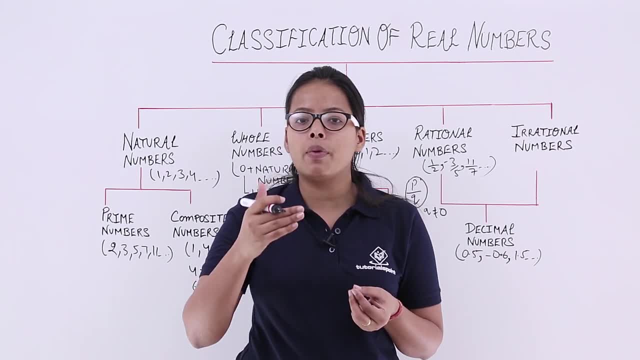 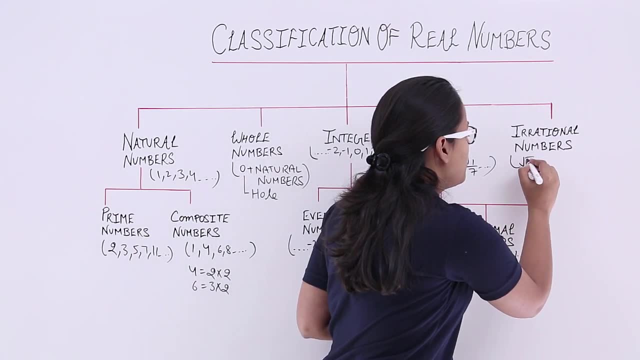 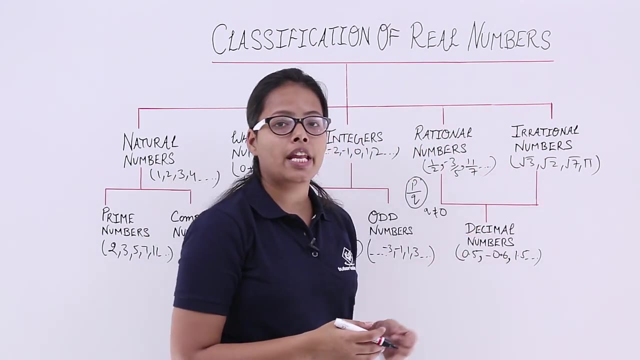 So those numbers which cannot be presented in integer, by integer fraction form, those numbers will come under irrational numbers. Let's see, for example, root 3, root 2, root 7, pi. All these numbers cannot be represented. Actually, there are infinitely many numbers. 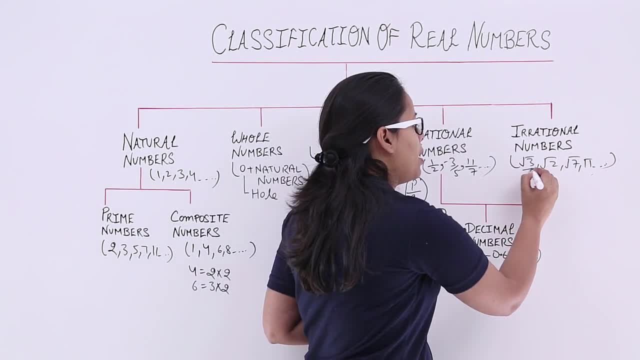 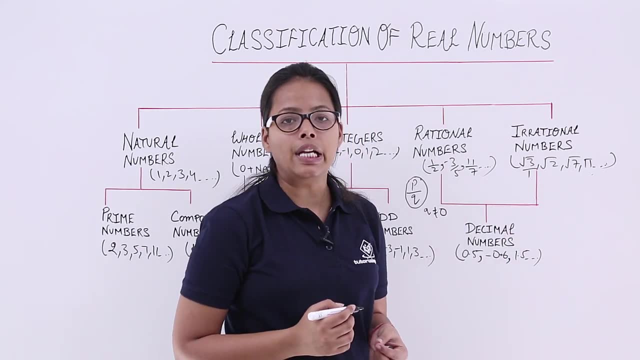 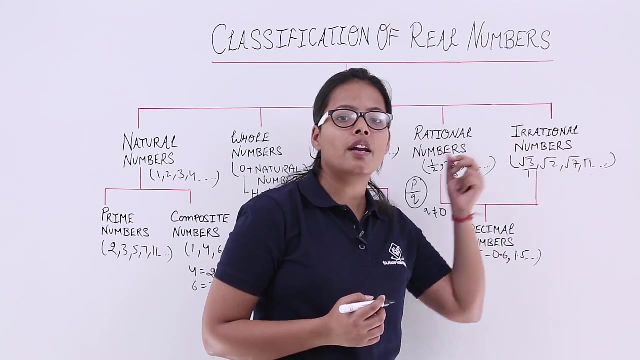 Okay, So you can see here that root 3 by 1, where root 3 is a decimal form, when you'll start solving for root 3 and 1 is an integer. So total form is not an integer by integer fraction form. That's why this number is an irrational number. So what do you understand by rational numbers? Irrational numbers are all those numbers which can be represented in integer, by integer fraction formOkay, So those numbers will come under irrational numbers. That's why this number here is an irrational number. So whether 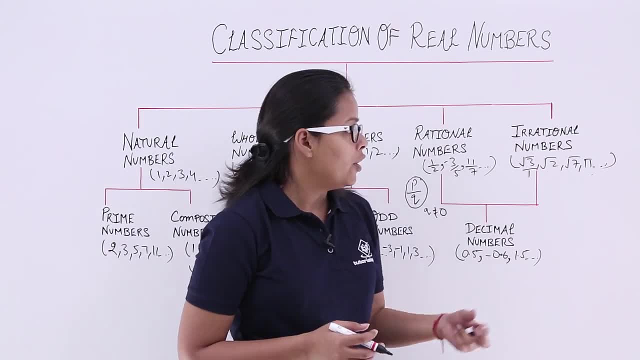 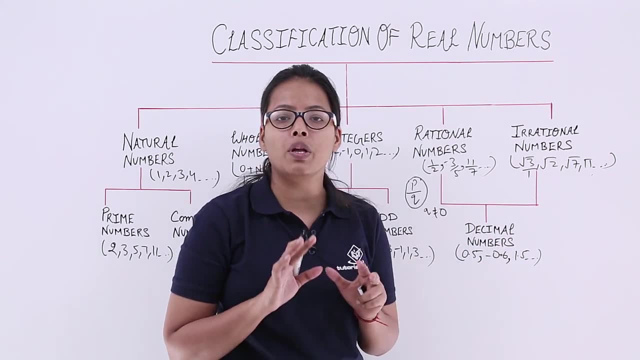 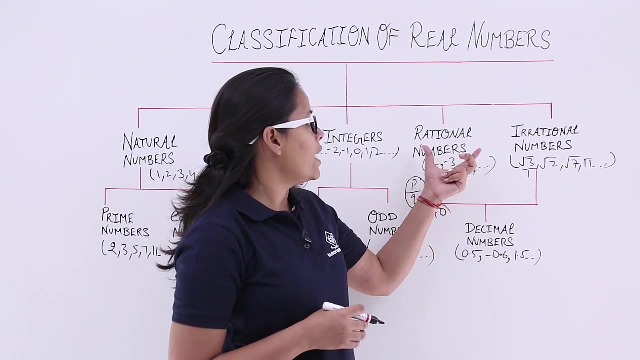 2 or any other number. It is less than or equal to 1.. All these numbers will痀ᴇ manuscript in announcer 2 pants those numbers respectively, so that there is definitely a decimal value. Okay, Now let me show you how the right side comes into view. 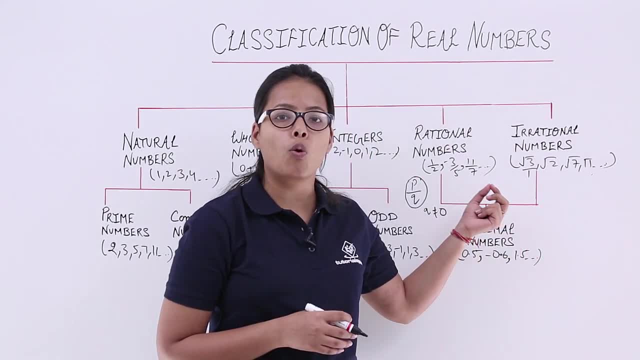 For example, we come here to this side. Okay, So you can see how we can make this. Bulgan method is differentさllä kut demorie kellah he DUquier zu bawz. it will appear 2or 3or. 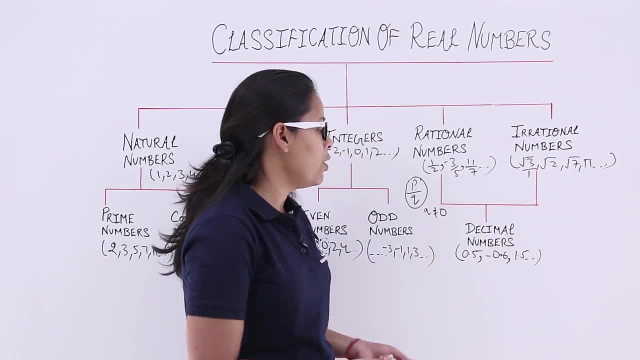 so on the left side, here is the rightmost positive. Now let's stew the present blunt. so by contribute receiver fv is equal 1 over voivert gizelnik anderer prayersE. So let's see what kind of decimal numbers you will get after the expansion of root 3. 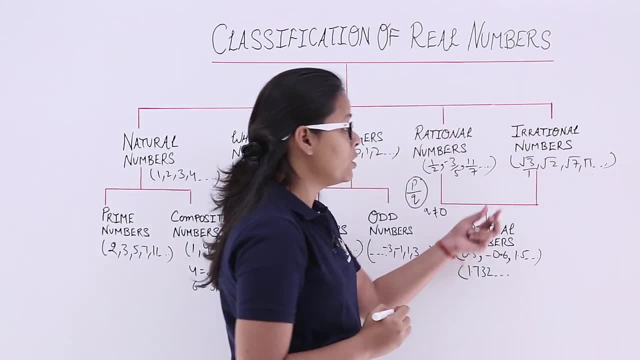 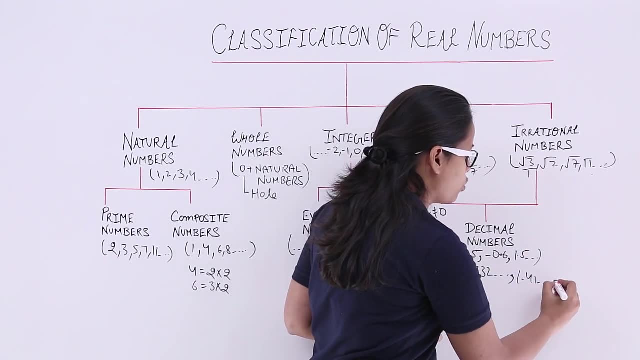 such as 1.732, so on, when you will start solving for root 3,. when you will start solving for root 2, you will get 1.41, up to so on. These decimal digits are non-repetitive in nature, Okay. 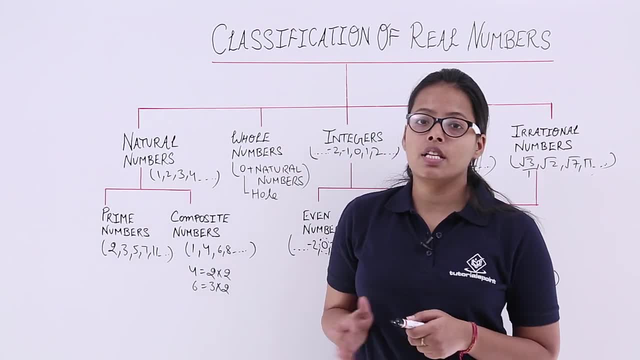 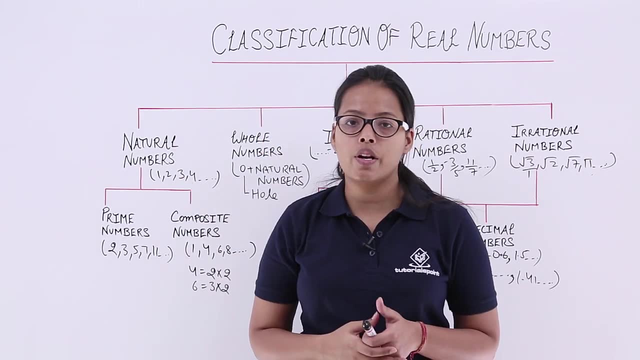 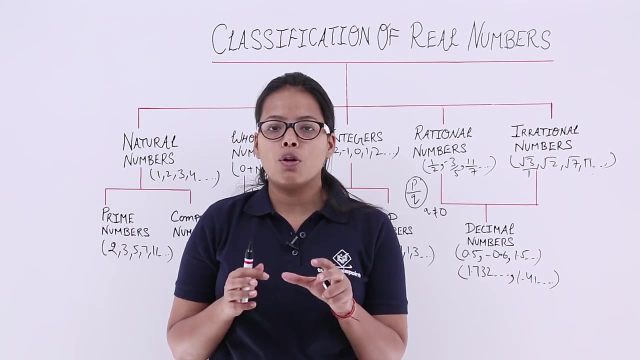 So let's summarize what we have discussed in this lecture. We have discussed real numbers, which is classified into 5 categories, such as natural numbers- All the counting numbers comes under natural numbers. Whole numbers: 0, including all the natural numbers, are the whole numbers.